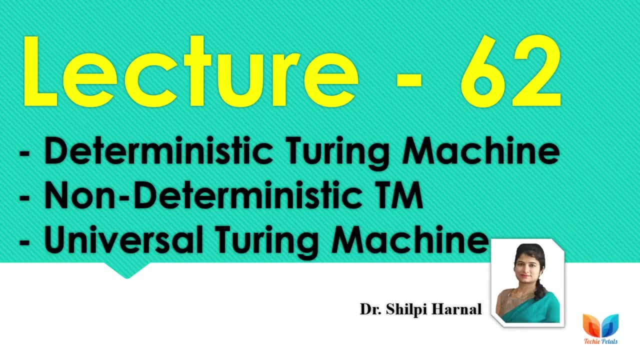 Hello everyone, so welcome to the next lecture. Hope you have practiced the Turing machine construction questions from the previous lecture. So here in this lecture we are going to start with some theory topics. that is, the deterministic Turing machine, non-deterministic Turing machine. 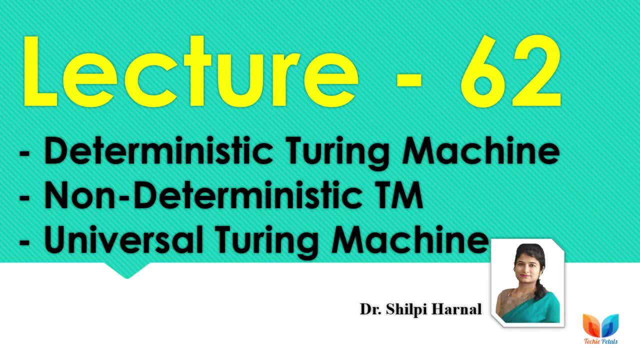 and the universal Turing machine or UTM. So all these topics- deterministic, non-deterministic Turing machine- are very much similar to the DFA's and NFA, and deterministic PDA- non-deterministic PDA- with a little bit of variation and different properties. So let's start with the lecture. 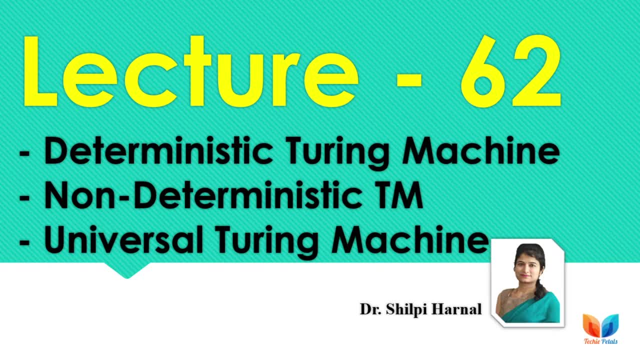 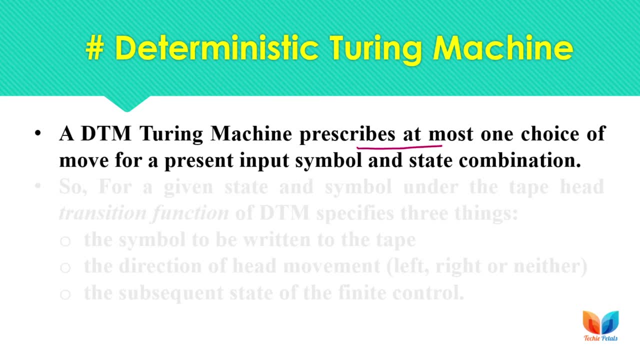 with a brief description of these topics and the examples. So here, a DTM or deterministic Turing machine prescribes at most one choice of move for the present input symbol and the present state combination. So from a state, from the present state for an input symbol. 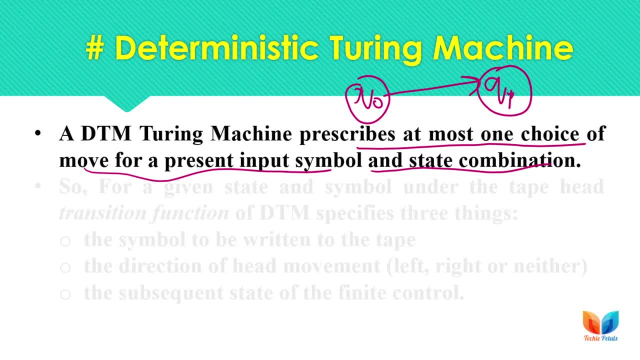 so from from, say, from Q naught or any other state for an input symbol, we can move to at most one state. only in case of Turing machine For a Q naught, for input symbol A we can have only one possible. 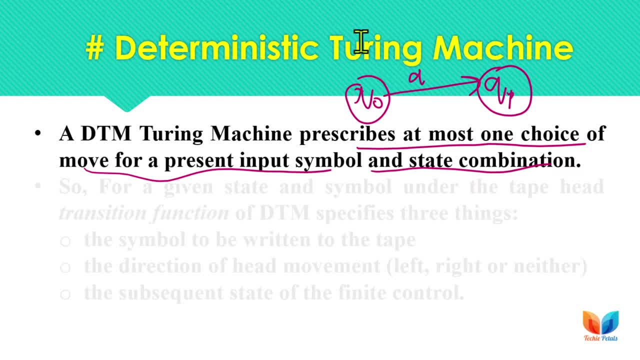 moves to any of the state, may it be to itself, But we must have only, at most, one combination of move. We may not have any other move, But if we are specifying the move, so Q naught and A will comprises of only one transition. Same way, Q naught, we can have only one transition. 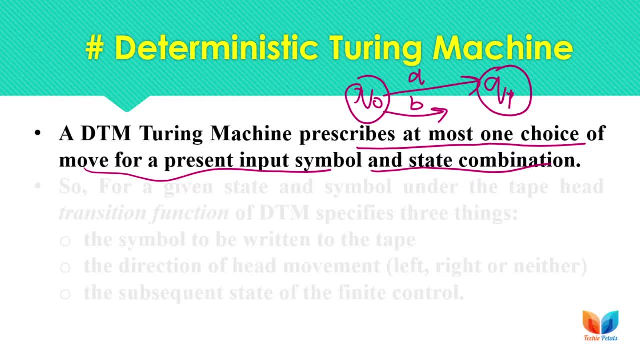 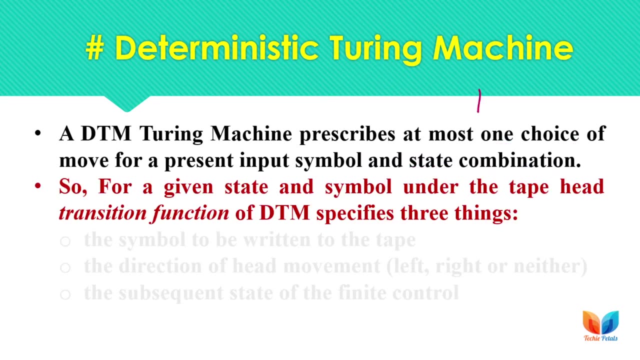 Same way Q naught for input. symbol B will also comprises of one transition, only at most one transition. So this property is exactly similar to the DFA. So we can say that if for a Turing machine we are reading the input from the tape, So from for a input tape. 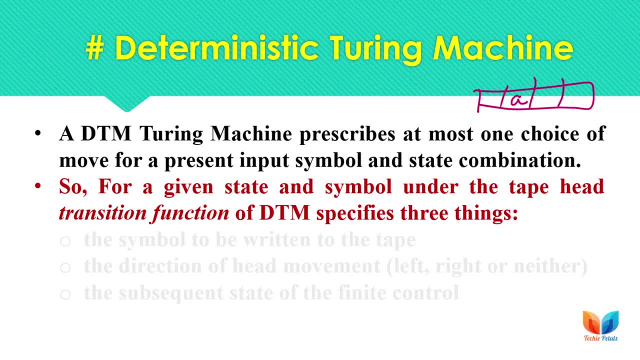 we are reading a symbol, suppose A and for a, from a given state. we are reading a symbol by the tape head. So tape head is presently pointing to this state. So we can say that tape head is presently pointing to this symbol. So every transition of deterministic Turing. 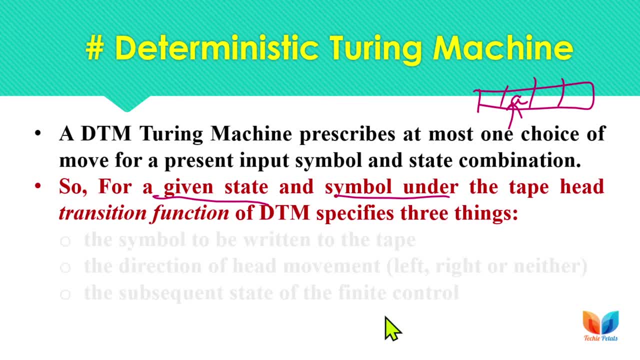 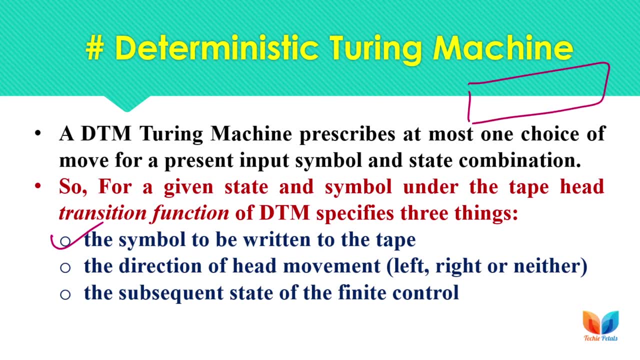 machine is going to specify these three things. So first thing is the symbol to be written on the tape. So we are reading, as we are reading, A from the tape. So after moving from any state, suppose we are at Q naught, So from Q naught, after reading A, we are. 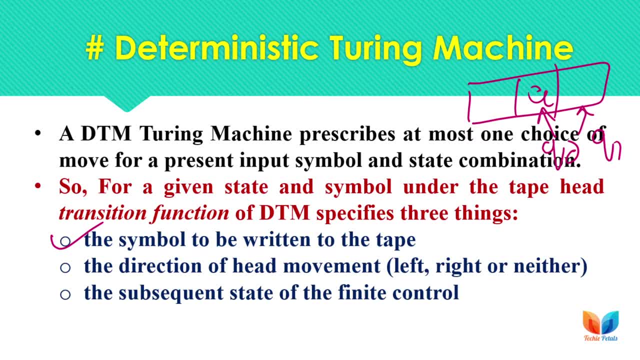 moving to say Q1.. Now we are pointing to the next symbol, but here we have only one move. So after moving from any state, suppose we are at Q naught. So from Q naught, after reading A, we have replaced this A with the capital A. So here the symbol to be written. 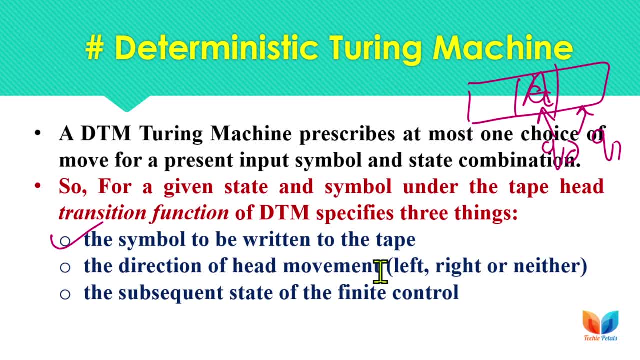 on the tape was capital A. The direction of head movement means next symbol to be read is from left or from right, or neither means. neither is the case where we are moving to the halt state: halt accept or halt reject. So this is the case of static move, where 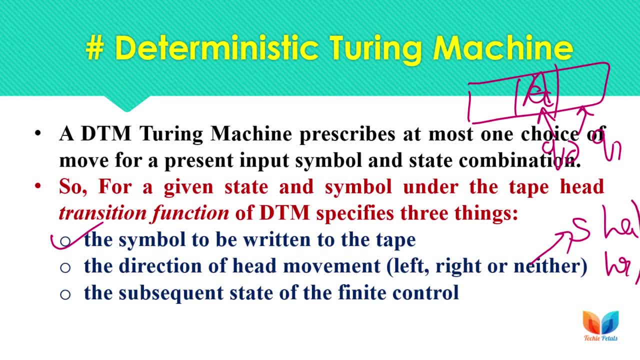 we were moving to the halt accept or halt reject state. any of these states. So left move or the right move, for the next symbol to be read from is left or right. So here the next move is to the right direction, as we are reading next symbol from the right and we will be. 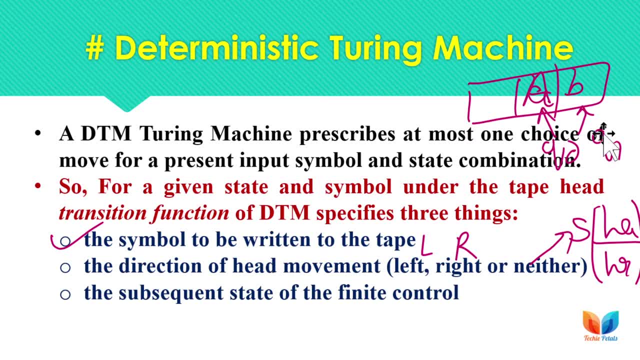 performing operation now from Q1 for next input symbol from the right. So the subsequent state of the finite control is Q1 now. So in this way, for every transition we are specifying these 3 levels. I am writing the desired value. So the further we go and we are going to write from the left, 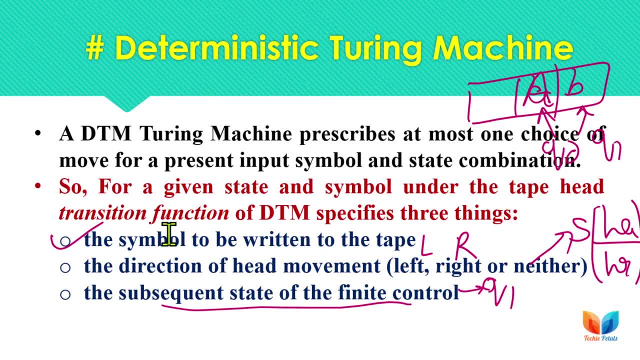 So here the next move is to the right direction, as we are reading next symbol from the right. these three things means the symbol to be written in place in replacement of the present input symbol that we are reading. and second, the direction of next head movement means either we will be reading the next symbol from left or 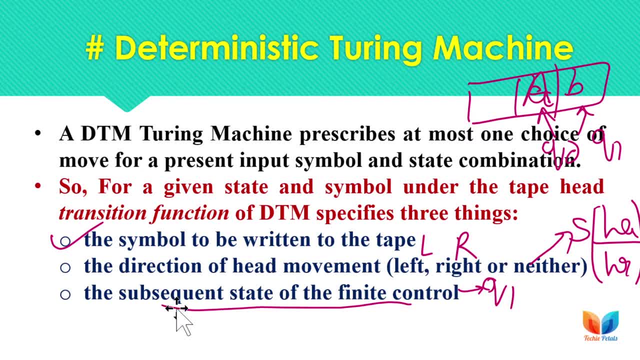 right. or, and the third thing, we need to specify the next state from which the computation will begin. so here, from Q naught, we are writing the symbol capital a on the tape and the next head movement is right. and also we will be reading the next input symbol from the next state, that is, subsequent state Q 1. so this is: 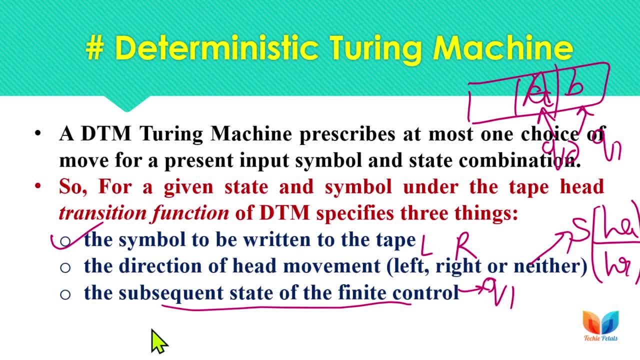 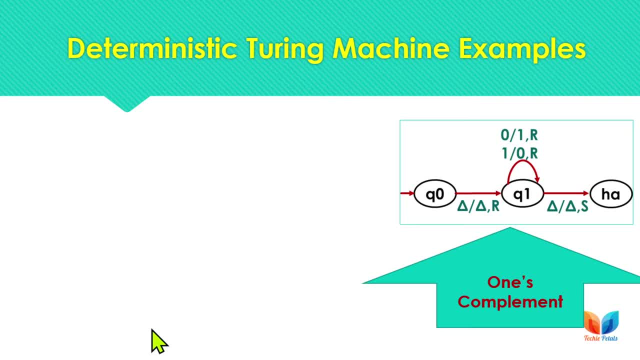 the way how we define the deterministic Turing machine and so far, whatever questions we have done, we say for the one's complement of binary number to convert all lowercase letter to the capital letters and for the palindromes. so all those questions were the deterministic Turing machine. 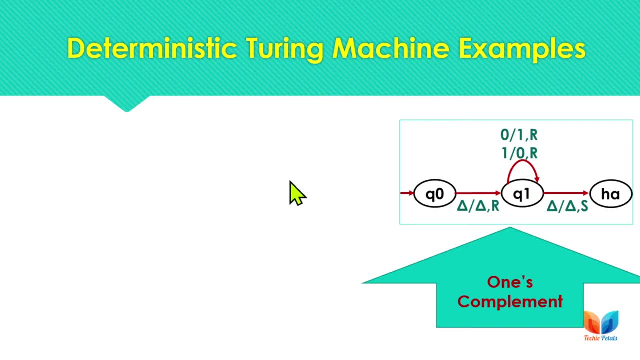 nor non deterministic Turing machine, as we were having only one choice of moved from��요 state for every input symbol. So all those questions were example of deterministic Turing machine. So here is the first example that we covered in the previous lecture, as once 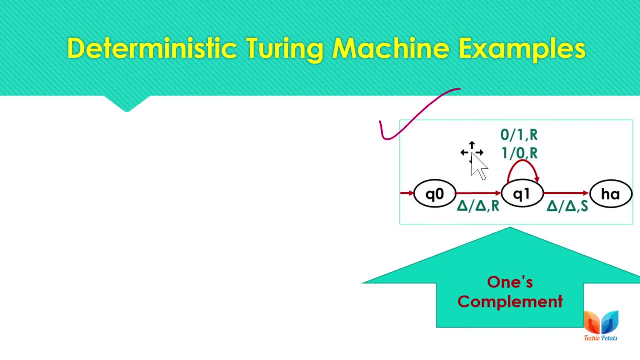 complement. So once complement. this machine will give the once complement of the present input symbol, will read the binary number from the tape and after the halt state- we are at halt state- the symbols on the tape will be representing the once complement right. So 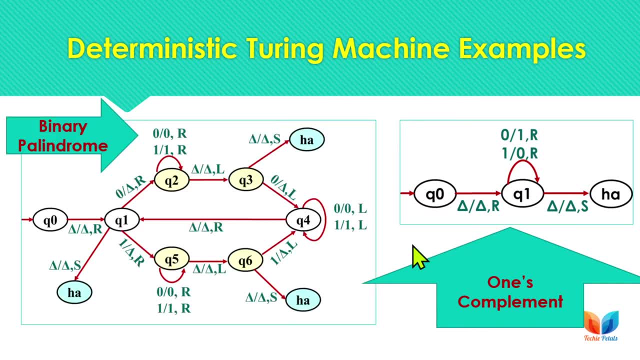 same way. two's complement question was also deterministic Turing machine and this palindrome question. this we have solved with the help of deterministic Turing machine. where we were moving from, we were cancelling out one symbol from the left- Suppose this was the palindrome- so we were making the first symbol from the left as blank and again we are moving to the. 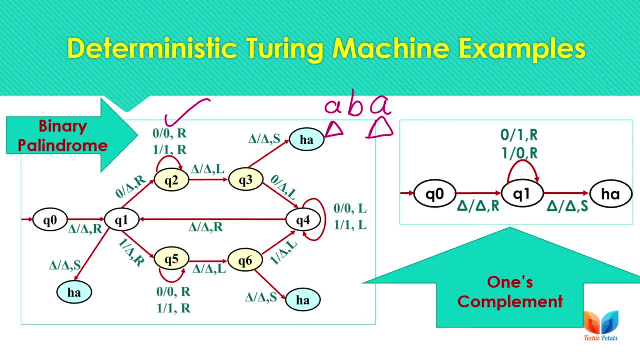 right direction and making the right most symbol to be replaced with the blank. and last we are. we were replacing this symbol, So in this way we were matching the symbols from left and right end. So, left most symbol with right most symbol. next, left most symbol with right most symbol. So all those symbols. 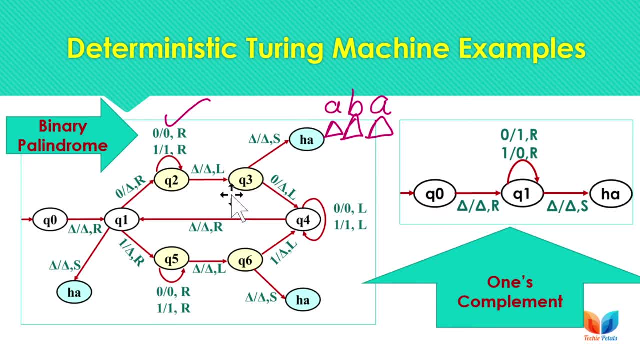 were matched and the string can be declared as palindrome or the non palindrome. So this was the question that we have covered in the last lecture. So all these questions are the example of deterministic Turing machine. So now let's check the non deterministic. 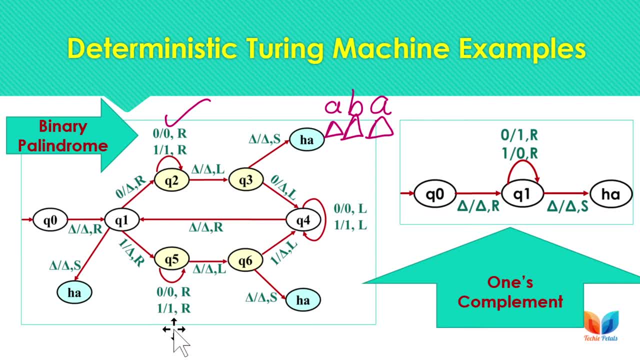 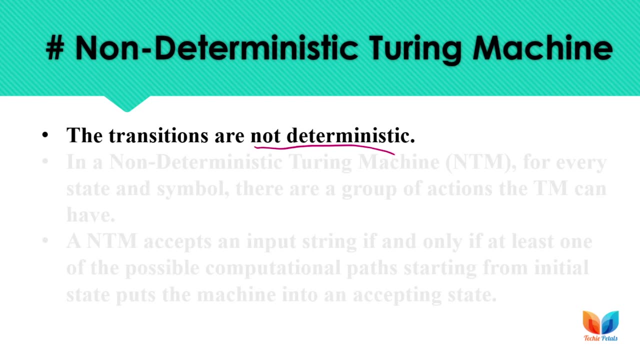 Turing machine like NFA. here we are adding the non determinism means from a state we can have multiple choice of move, as in deterministic we can have at most one choice right. So here is a definition. So transitions are non deterministic. that is very well understand. 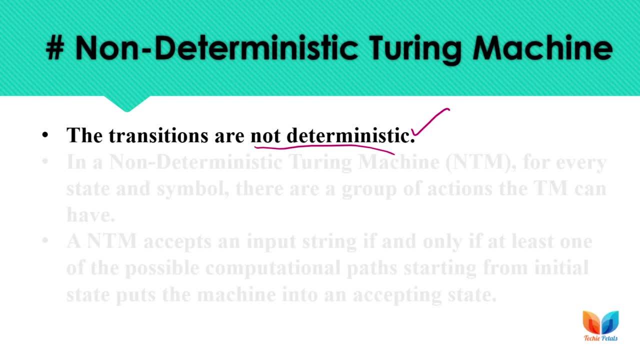 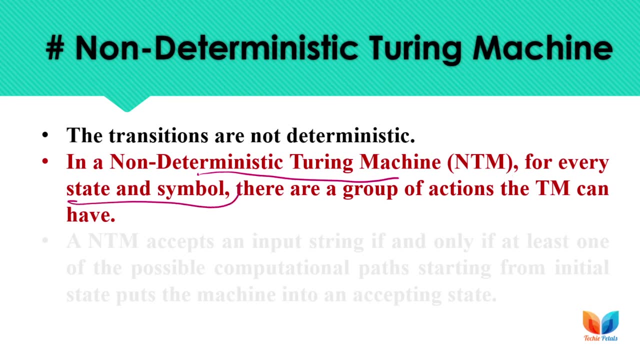 that all the transition for non-deterministic Turing machine are going to be non deterministic only and in a non deterministic Turing machine symbol. so now for every state and symbol combination, like NFA, there can be a group of actions that a Turing machine can have, means we can have multiple transitions for a state and symbol. 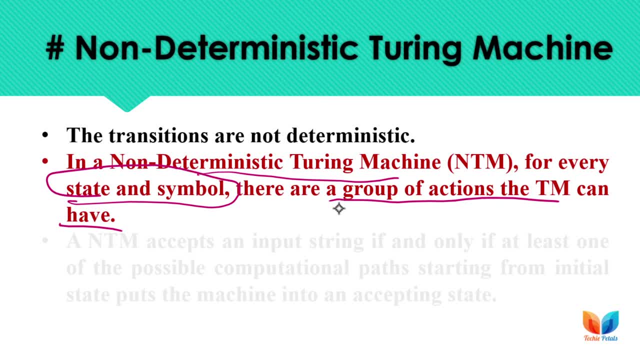 combination. okay, so, like NFA, from the starting state Q0. after reading the state, we are going to have multiple paths. so one path ending at Q1, another path ending at Q2, another path ending at Q5 and, if any, one of the path. so these are the path, not the single states. so 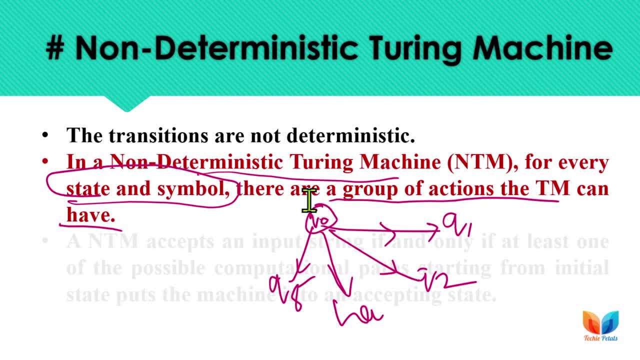 if any of the path after reading the input string from initial state ends with the halting state, then we can say that the string is accepted, or we can say that the output is on the tape means computation is complete. now you can read the output from the tape, but if none, 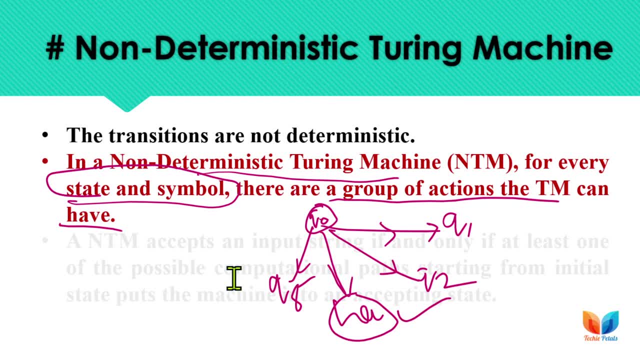 of the path leads to the acceptance state, Then the input string is accepted, Then the input string is rejected by the non deterministic Turing machine. so this phenomena is same as a non deterministic finite automata, NFA. so here is the rule. so NTM or non deterministic. 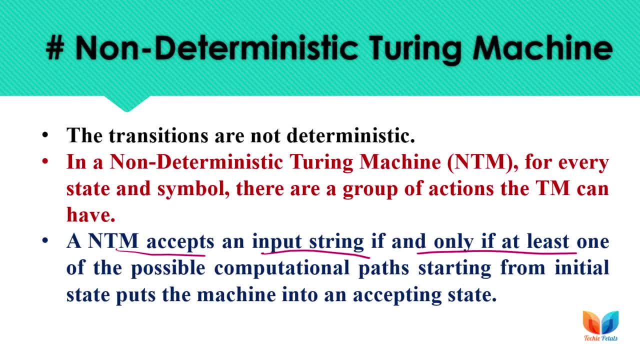 Turing machine accept the N input string. if, and only if, at least one of the possible computation path starting from the initial state puts the machine into an accepting state, then we can say that the machine, the input string, belongs to the N input string. So the input string belongs to the language. otherwise the language is string is not according. 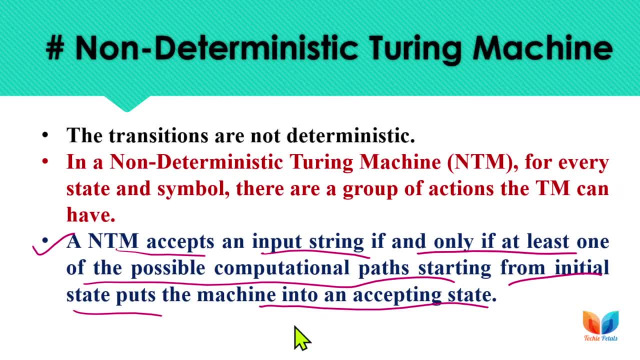 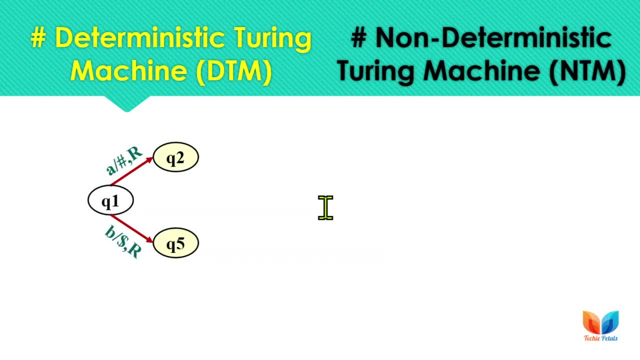 to the language of the Turing machine. So this property is exactly similar to the non deterministic automata. So here is the example of deterministic Turing machine. here from Q1 we are having one move for input symbol A to the state Q2, and from Q1 we are having another move for input symbol. 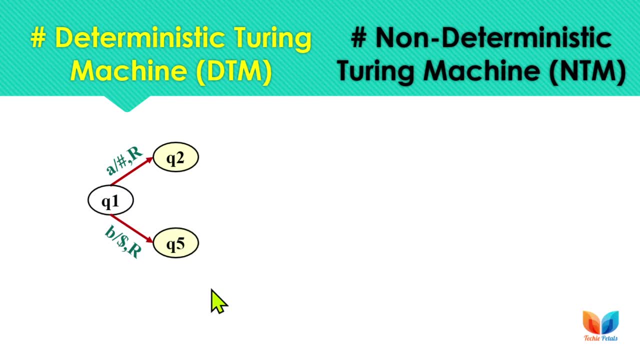 B and we are moving to the state Q5.. For the first case, we are replacing the symbol on the tape, as we are having the symbol as B or A. ok, so as we are having A, so we are replacing the present symbol A with hash and. 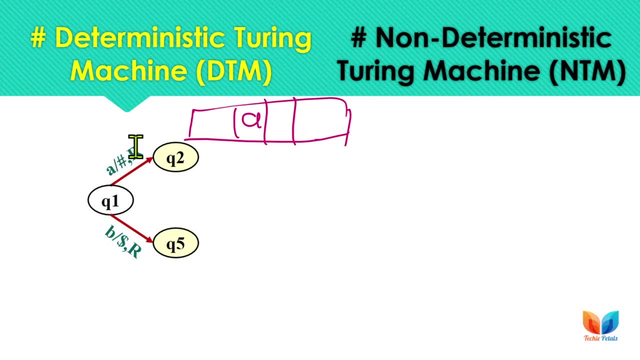 next move is right means head movement. next required head movement is from right. so here we are replacing this A with hash and moving to the next symbol. ok, suppose next symbol is B. So we are replacing B with the dollar symbol and moving to the right right. 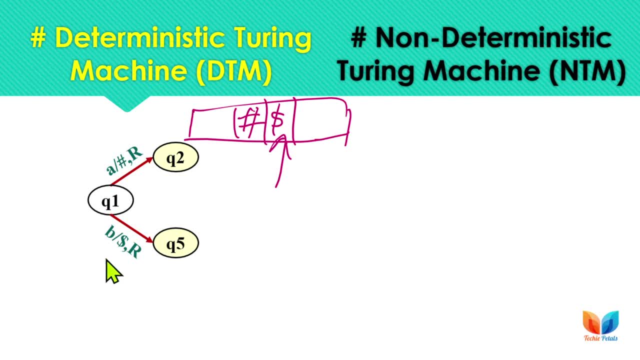 So this is the way how we are performing operations with the Turing machine. So we read A and replaced it with hash and move to the right. Now, if we are having the same move from the Q to for B, we replace it with dollar and move to the halt state, say: 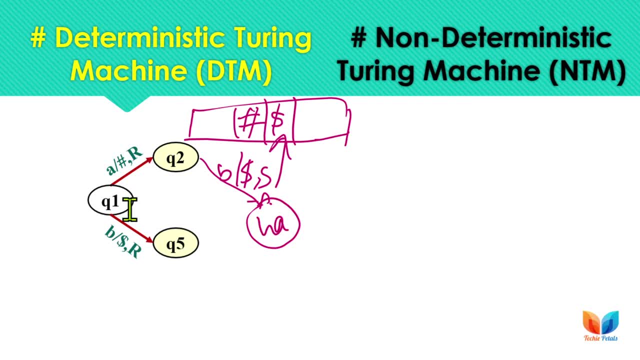 We are showing the acceptance here, So halt accept state is here. So after reading B from the Q to, we are replacing it with dollar and moving to the halt state means accepting state. So deterministic Turing machine is having only one move for one input symbol from the present state, from a combination of input symbol and a state. 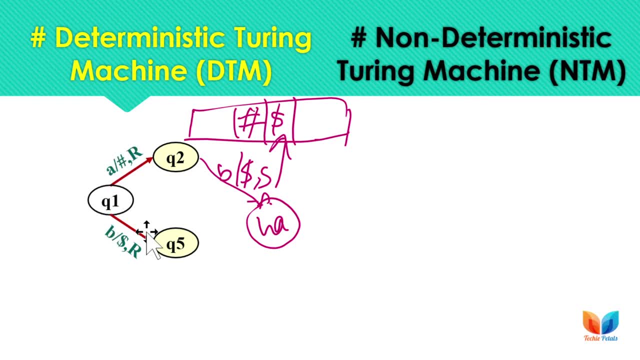 Next here, dollar and hash are the tape symbol, So do not get confused with this symbol. We can have any other symbol to be replaced or write on the tape. So you can use any symbol: hash, blank, dollar, star, anything to be replaced on the or to be used for the computation as tape symbols. 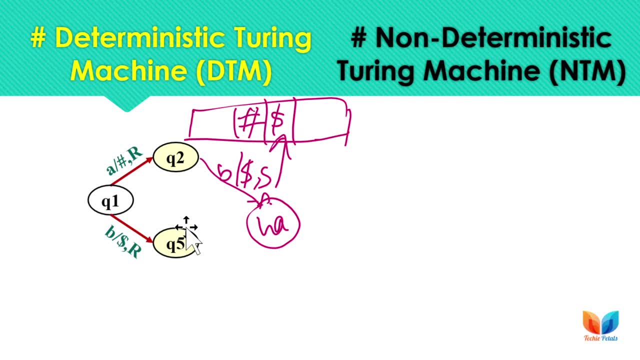 We have discussed this concept in previous lectures also. So you can use any symbols as per your requirement, as per the need of the question. Now, if we have the non-deterministic Turing machine, then we can have multiple choice of move. Say, here we are having one move for input, symbol A to the Q2.. 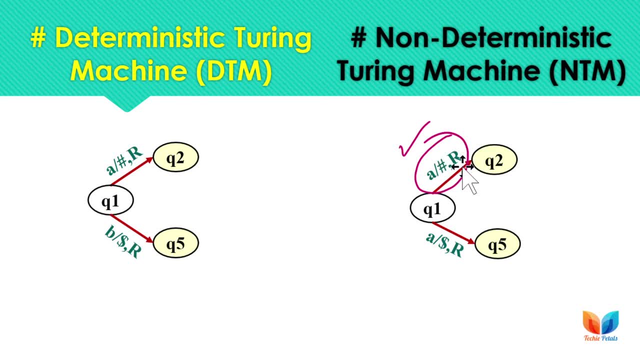 But here we are replacing A with a hash and we are moving to the state Q2. and same way from Q1 for the same input symbol A. we are having another combination. So Q1 for input symbol A, we are replacing it with dollar sign and we are moving to the state Q5.. 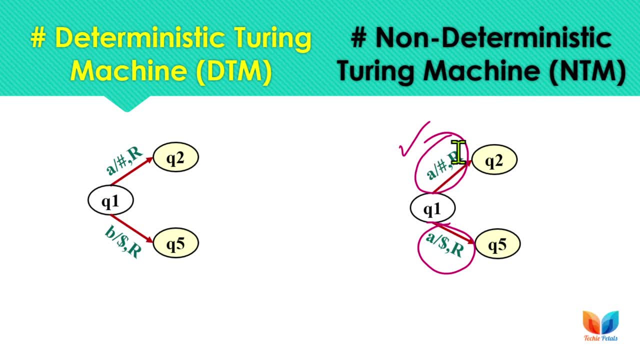 So for a input symbol we can have two transitions here. This is not possible with DFA, but yes, it is possible with NFA. So this is the main property of non-deterministic Turing machine or any non-deterministic machine. So here we can say that deterministic Turing machine as NTM comes in the outer section and DTM comes in the as a inner circle. 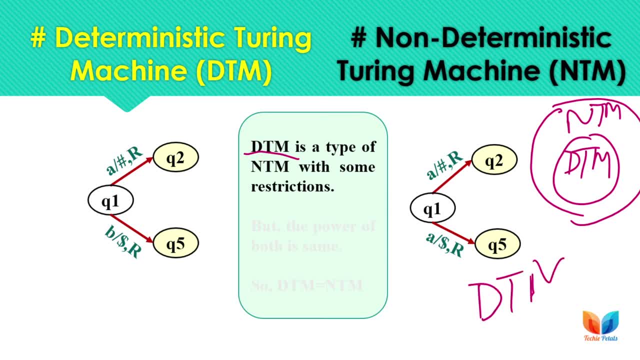 So we can say that DTM is deterministic Turing machine, is subset of NTM, like NFA and DFA, So as NFA, So we can say that deterministic Turing machine is also subset or the part of the NFA, or deterministic Turing machine is also NTM- non-deterministic Turing machine, with some restrictions. 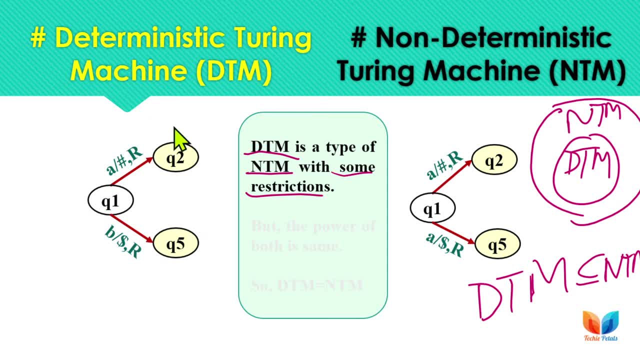 So here all the properties are same as non-deterministic Turing machine. just we are making some restriction that we can have only one move for one input symbol and one combination is allowed. at most one move is allowed, So all. So now something more focused that we can say that with these restriction we can say that every deterministic Turing machine is also non-deterministic Turing machine. 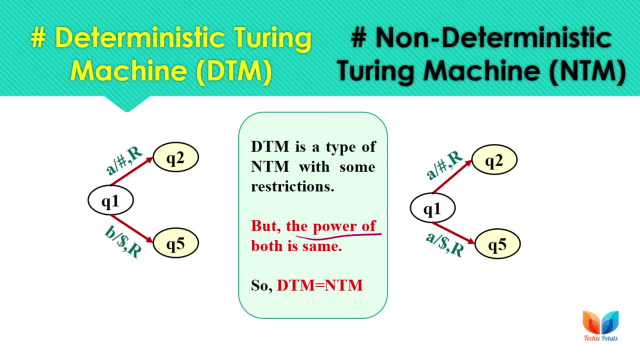 But the power of both is same means. whatever we can achieve, this deterministic Turing machine we can also achieve with NTM, and universe is also possible. So here the power of deterministic Turing machine and non-deterministic Turing machine is same means one. question v. 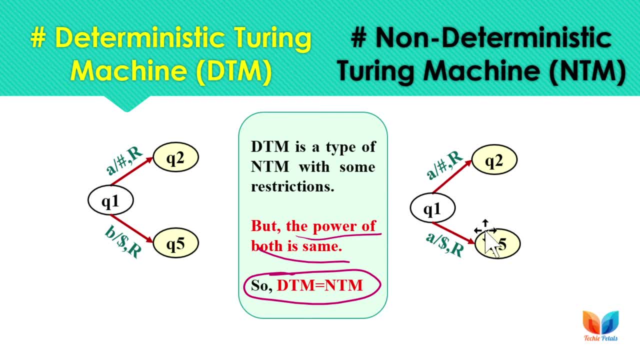 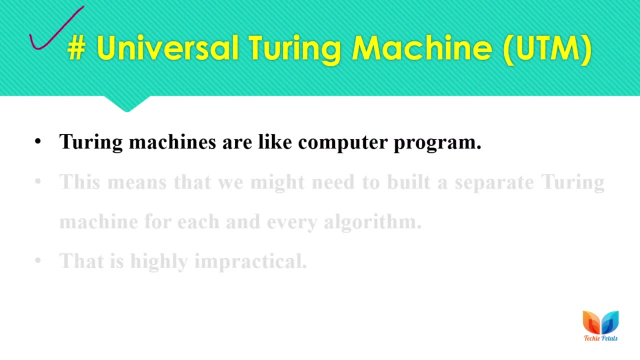 A can be solved with If a, If a Turing machine, it can also have the solution in deterministic manner. so here we can say that both the power of both machines is same. next we have the concept of universal Turing machine. now you can thank universal Turing machine. 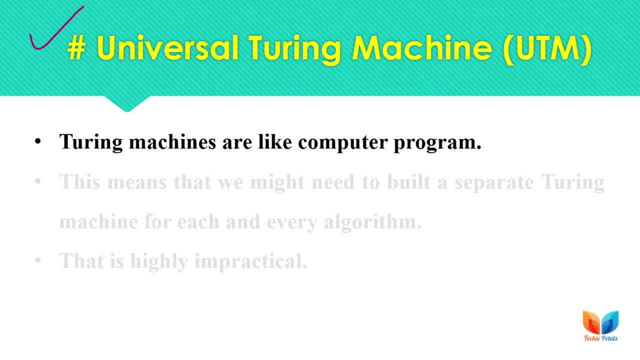 as a computer that can solve any problem. okay, so we are expressing Turing machine like the computer program, so one Turing machine is equivalent to one computer program, right? so we are assuming this now as one program can perform only one task, right? so if you have written a program in C language or in any other, 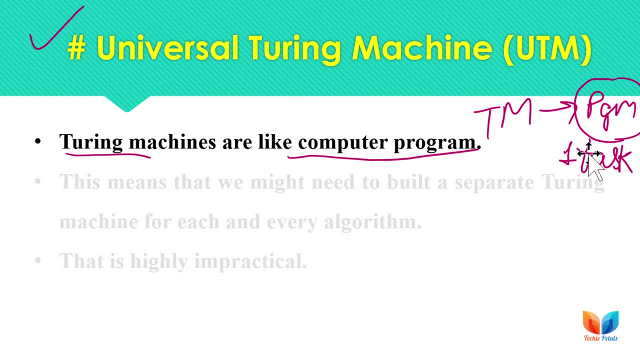 language to perform the addition operation, then it will perform addition only. and if we have the program to perform multiplication or to calculate area of the circle, then it will perform that task only. so one program is performing one task. same way one Turing machine is capable performing one operation only. suppose i have designed the turing machine to check the palindrome. 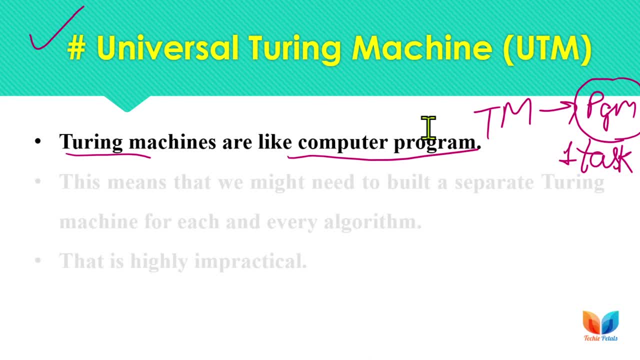 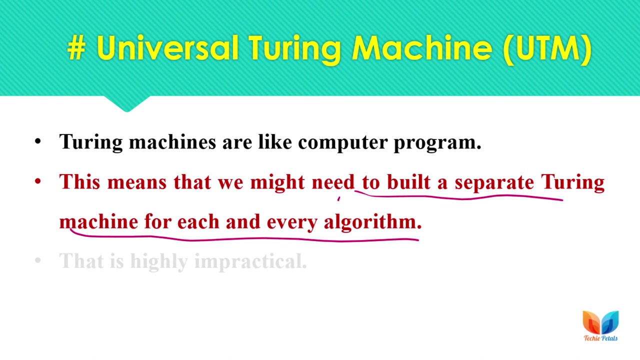 or to multiply or to perform addition, so that turing machine will perform that fixed operation only. we cannot, cannot expect multiple operations from a turing machine. this means this means we might need to build separate turing machine for each and every algorithm. so if we have to perform 10 operation, thousands of operation, so is it possible to build? 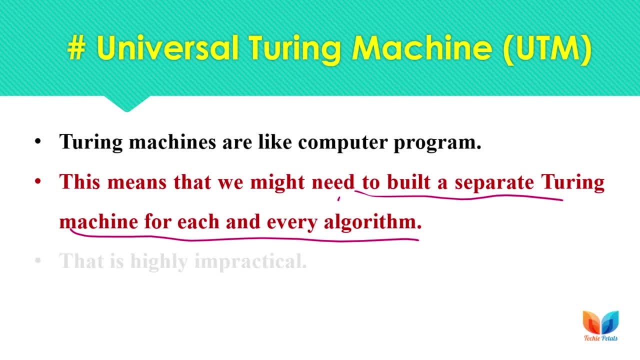 different turing machine for every operation. so we can say that this approach is highly impractical. means we cannot have any number of or multiple number of turing machine for every problem. like we have a compiler, so a compiler for the c language or any interpreter for any language. 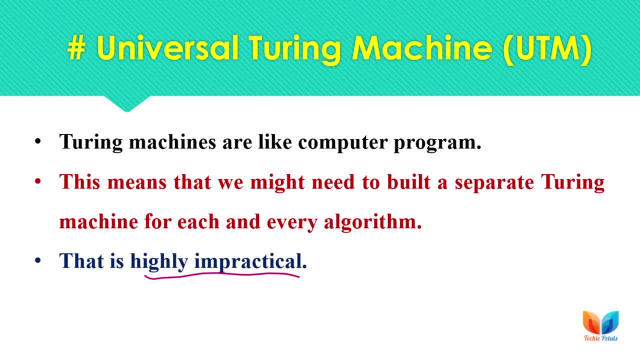 so that compiler or that interpreter is capable of running any program of that language, so same way we must have some mechanism or some machine that can, that can, perform all the operations. means every turing possible, turing machine, possible algorithm should be implemented in one machine, only one computer, so one machine that can have the power of all turing machine. turing machine. 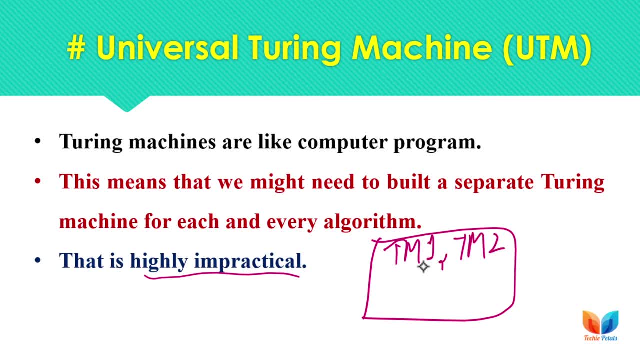 one suppose turing machine two, so one machine that can perform the action or the perform the outputs of any or any possible turing machine- and if such machine is possible- we are calling it universal turing machine- that can operate or act as any of the turing machine right. 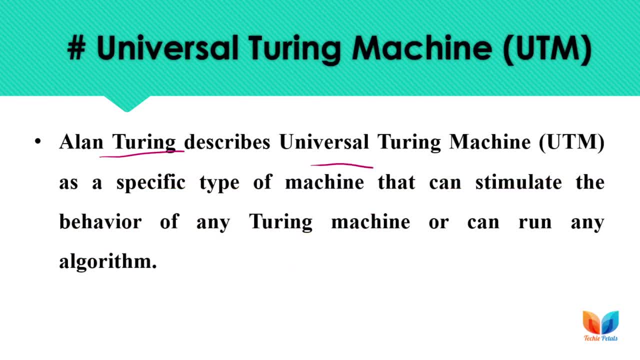 so here we can say that allen turing describes universal turing machine as a specific type of machine that can stimulate the behavior of any turing machine and can be capable of running any algorithm. as we have described, universal turing machine is described in a form that can run any algorithm can. 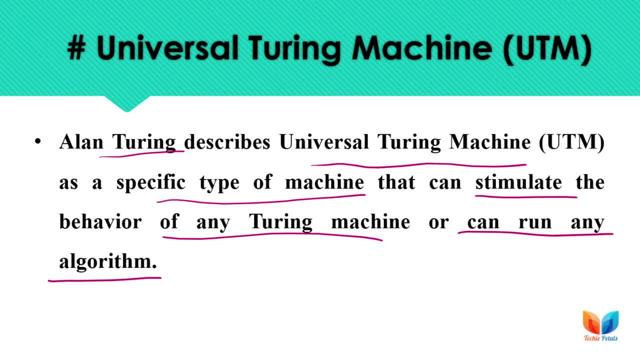 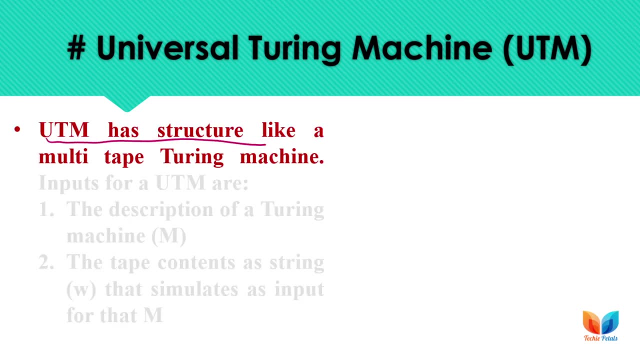 can be connect as any turing machine can show the behavior or stimulate the behavior of any turing machine. so this is the concept of universal turing machine. let's discuss this with a example here. so utm structure or the universal turing machine structure can be taken as multi-tape turing machine. 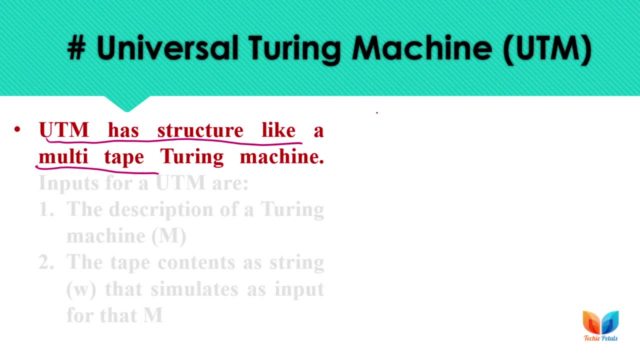 so by multi-tape turing machine we we mean that we have one machine. suppose we have one turing machine, m, so we are taking it as m only, so machine is named with m. now the question that we have done so far? we were having only one input tape. 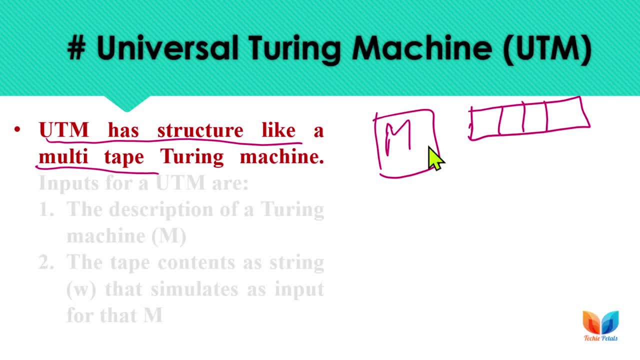 okay, right, so we were reading the input from the same tape and we were writing the output on the same tape and if the recognition is required, then we were moving to the halt accept state or halt reject state according to the input strength given. okay, so now let's take the example of 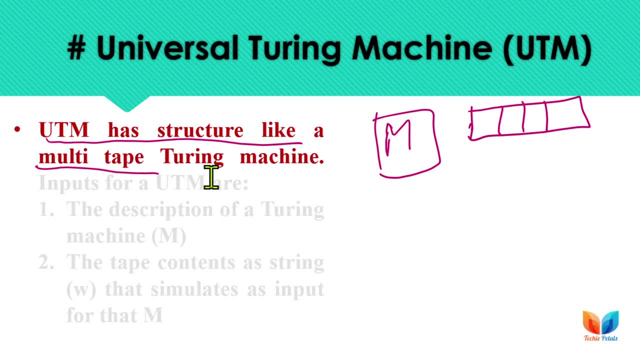 multi-tape turing machine. by multi-tape turing machine, we mean that we can have multiple tapes associated or linked with one machine. okay, that's why we were saying that the power of Turing machine and deterministic Turing machine is same. So what non deterministic Turing? 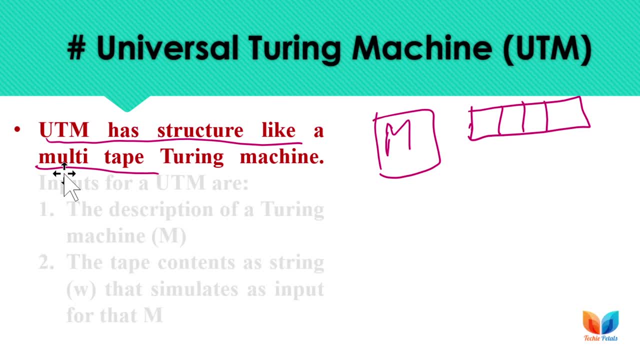 machine can achieve Deterministic Turing machine can also achieve with multiple tapes. So we can have the concept of multiple tapes with Turing machine, like here, let's suppose with single tape, as we have ABA as palindrome input string, So we were checking the palindrome. 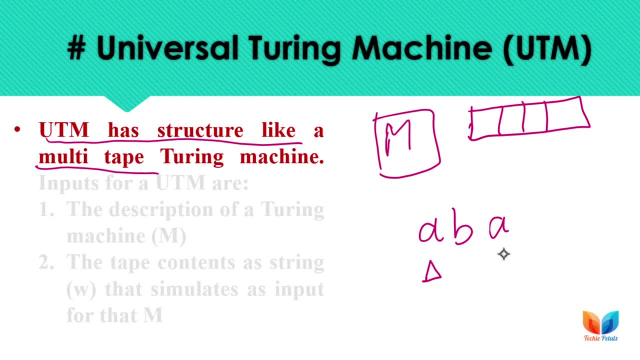 by cancelling out left most symbol with the right most symbol. by cancel we mean that we were replacing the symbol with a blank. So we were replacing the left most symbol one time and the second time we were replacing the right most symbol with a blank. So this: 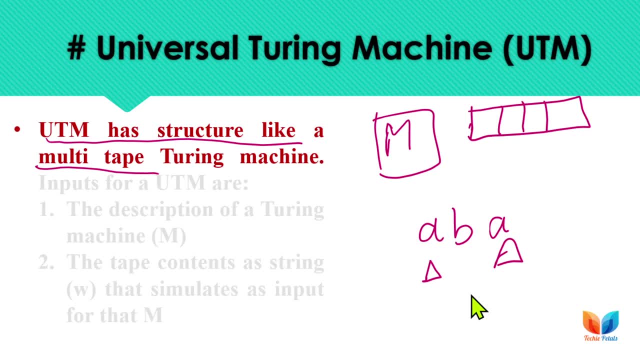 was our approach to deal with the palindrome string. So for this performing this operation, we were moving from. one time we were moving from left to right, next time we were moving from right to left, and next we were moving from left to right, And So on. So we need needed to move left to right, right to left so many times depending. 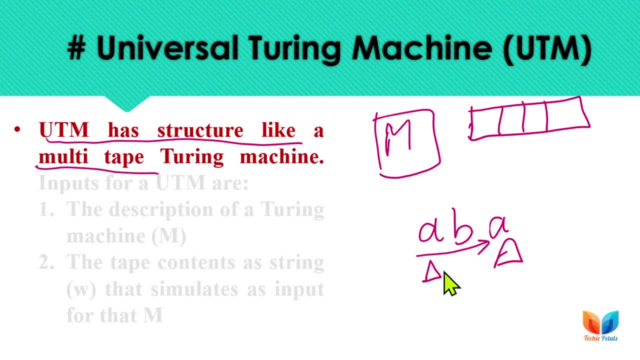 on the input string. So here is a different approach if we have multiple tapes associated with the or linked with the with one machine. So how can we solve this problem? with simple performing the one one time track means either from left to right and one machine is moving. 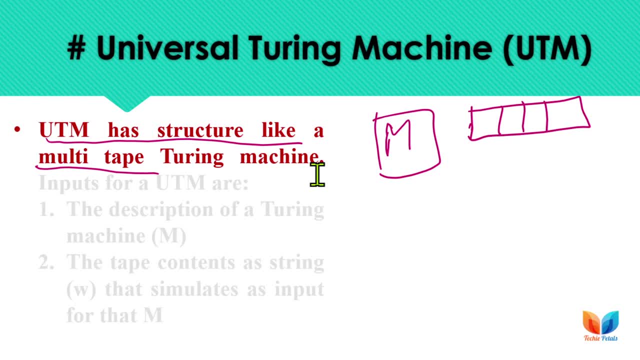 from right to left and we can easily check or recover, Check or recognize the palindrome strings, like suppose we have the same string here, A, B, A, over the input tape one and the second tape is also carrying the same input. I am just discussing the concept of multi tape Turing machine. if we have multi tape Turing, 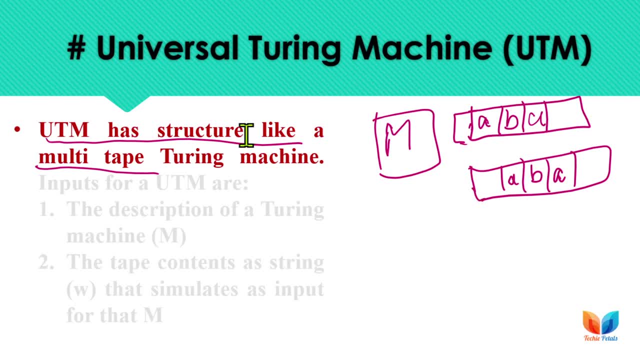 machine how we can make this operation to be done very easily. So suppose first Turing machine. So here the first tape, this is the second tape and one tape for first tape we are moving from left to right. So this tape is capable of moving from left to right and we are having 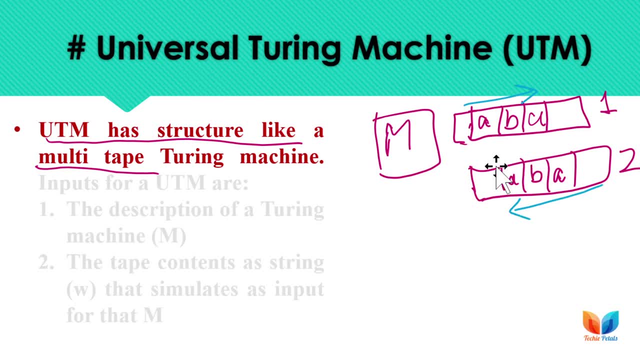 this tape where we tape, where we are moving from right to left. So here the right, where we are moving from right to left. and one for tape, one we are moving from left to right. So here for this tape. our tape head is pointing to the first. 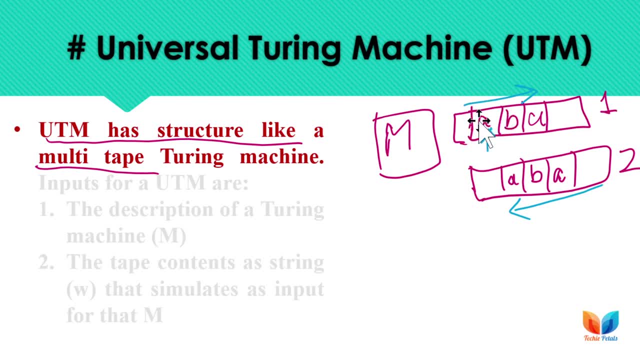 left, most symbol. ok, Once the machine is started and initiated, we are pointing to the first symbol for this tape. and as here we are moving from right to left, So for this tape, so for this tape we are moving from right to left and this time, for the first time, we are pointing 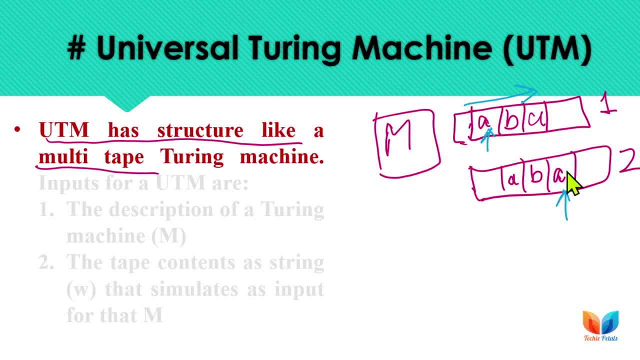 to the right most symbol, So we can easily match the symbols at the head of both tapes. ok, So I am just giving you the example how multi tape Turing machine can work. So here, after making this symbol from the blank and this symbol from the blank, or you can simply: 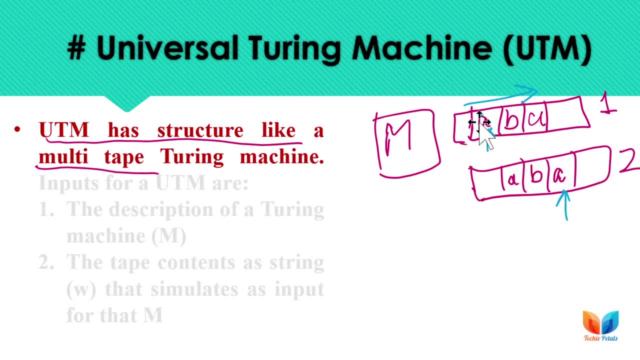 match if these symbols are same means tape head of first tape and tape head of second tape. if they are having the same symbols, then we can move to the right here and here we can move to the left. ok, and next symbol must also be same. next symbol must also be same. 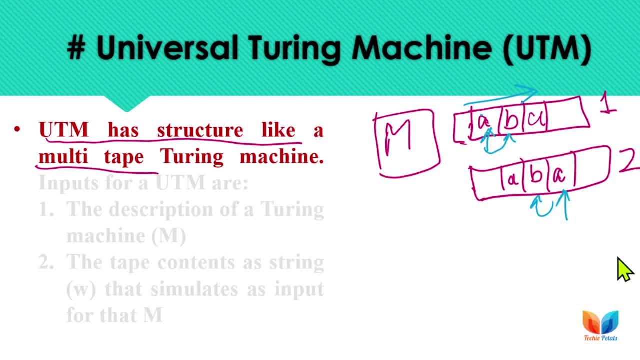 we must have the same symbol here and next the symbol again. we are moving to the right and we are moving to the left. So in this way we can easily check: by one by moving in the right direction and for the second tape by moving in the left direction. So this: 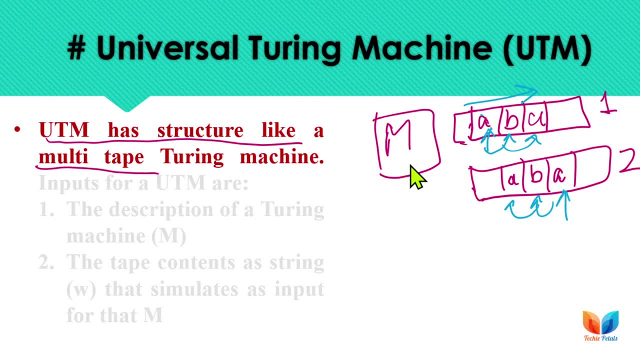 approach can help us to perform the operations easily. that is why we are saying that the power of deterministic Turing machine is same as non deterministic Turing machine, where we can have multiple moves with multiple tapes- ok. but for the implementation point of view we are not going to implement any such machine where we are reading the input from multiple 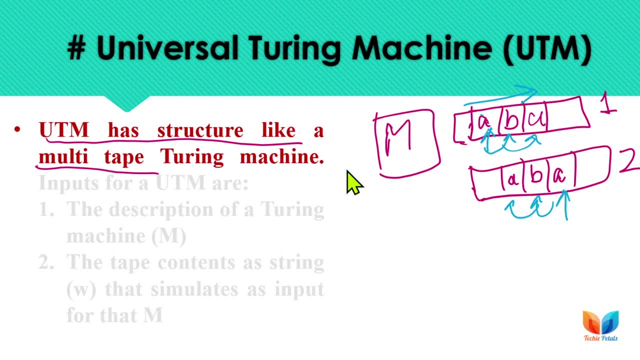 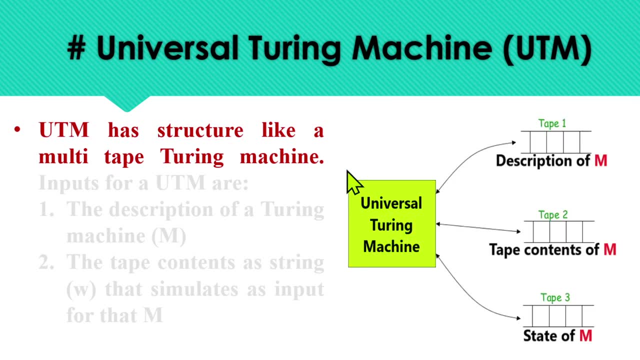 tapes and writing the input to the multiple tapes. but you have theoretical topic of multiple Turing machine. So we can say that the possible inputs for the UTM or Universal Turing Machine are: description of the machine means- Universal Turing Machine. Universal Turing Machine can act as any of the machine means can perform any algorithm. 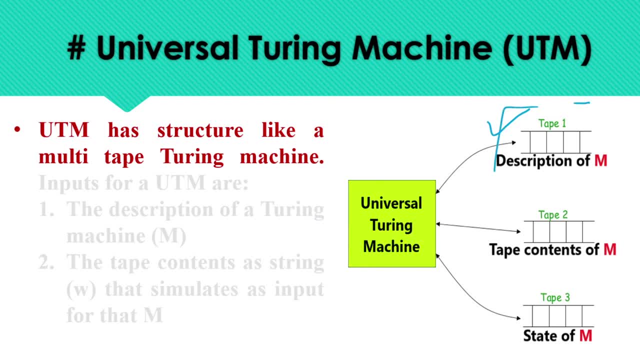 and can give the result. So, first of all, we need to provide the Universal Turing Machine with the description of the machine. suppose we want to perform addition or we want to perform multiplication. So the same same information we must provide to the Universal Turing Machine. ok, So, as it can act as any Turing Machine. So what operation we need? 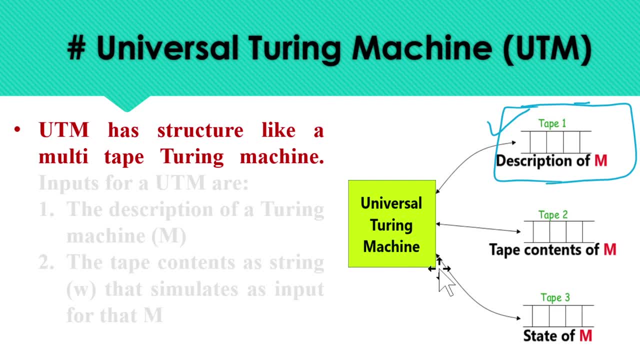 to perform at the particular time. we need to provide that description. suppose we want to perform addition, we want to check palindrome, we want to perform multiplication. So the same information is providing to the Universal Turing Machine and the second tape. second tape may carry the string. suppose we have to check W, for this machine means we have 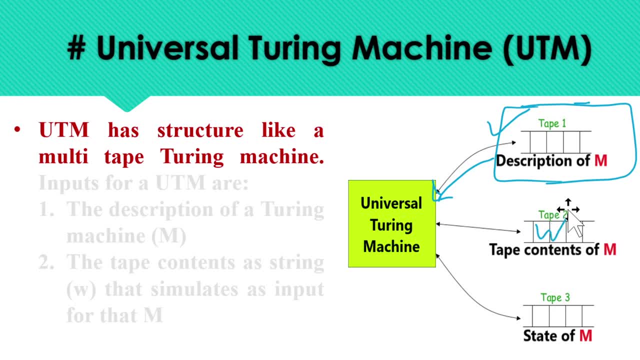 to check that W string is palindrome or not. So the tape one will provide the description of the machine that we have to check or recognize the palindrome string and the tape two is carrying the possible input string means the input is at tape two. the description is at: 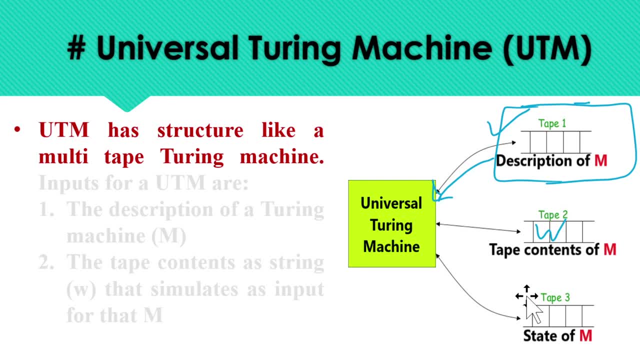 tape. tape one and tape three may carry the result, ok. or tape three may also carry the same input string, if required. or tape three can also carry the output. So, as per the requirement, as per the computation is required, So accordingly we may also carry the same. 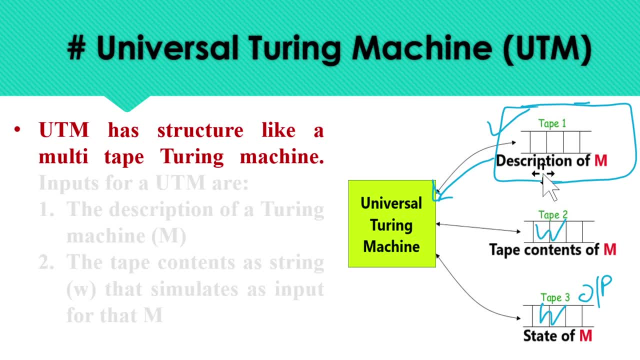 number of tapes, or we may have only two tapes, we may have three tapes, So this will depend on the requirement and the question. So Universal Turing Machine, as per the input, can perform the computation and can give the output. So here we can have the concept of multi multiple.